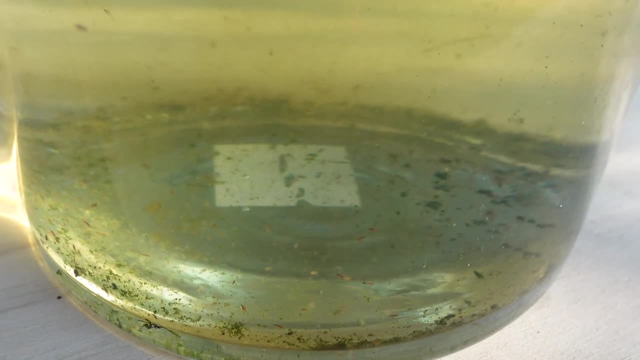 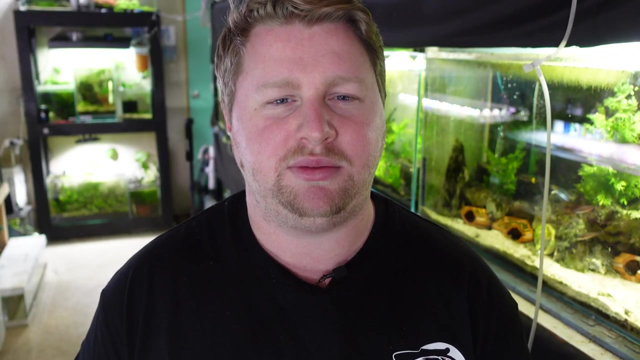 most bodies of water in the world, you can find wild Daphnia. This is really great because, although a lot of our fish in the aquariums are captive bred, some of the wild types and some of the more hard to feed fish will be used to eating. 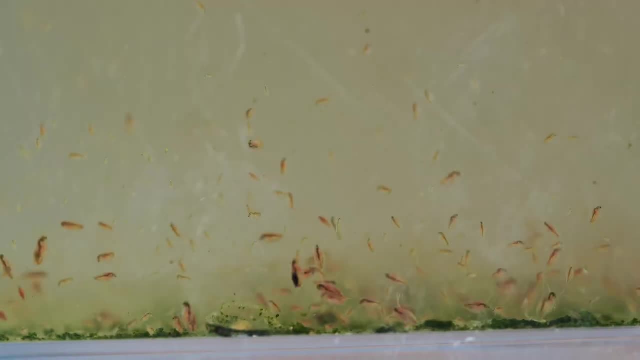 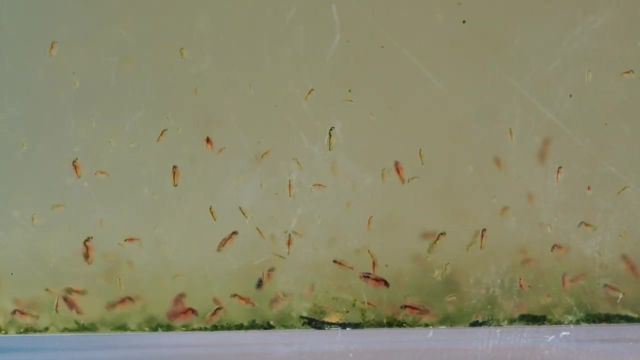 things like Daphnia in the wild. so it might be that last key that you need to unlock success keeping a really tricky fish. Other than that, any of the more common fish you know- guppies, platys and other communities- will be able to feed Daphnia. So let's get started. 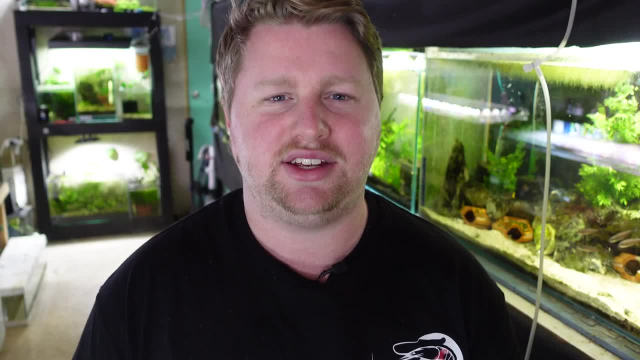 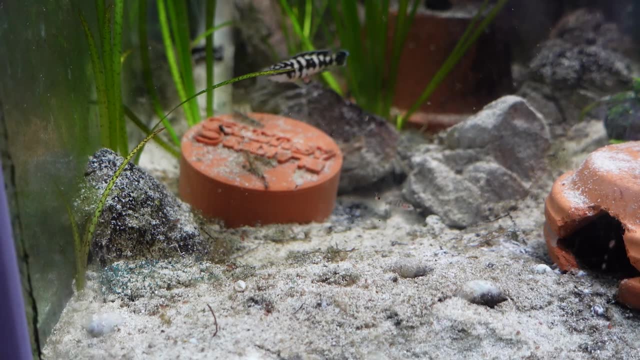 Fish will really love Daphnia as well, and everything just goes crazy for the hopping motion that they exhibit in the water. Daphnia are commonly referred to as water fleas, and that's because their body shape is very similar to common land fleas. 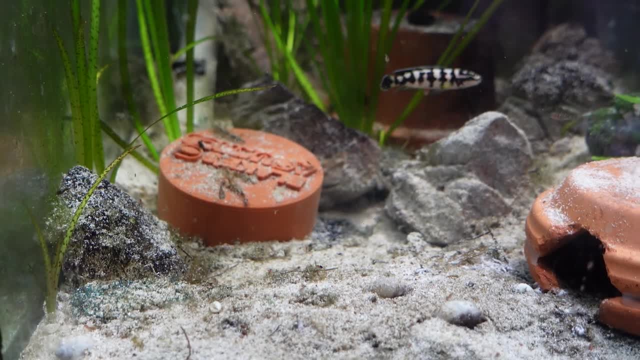 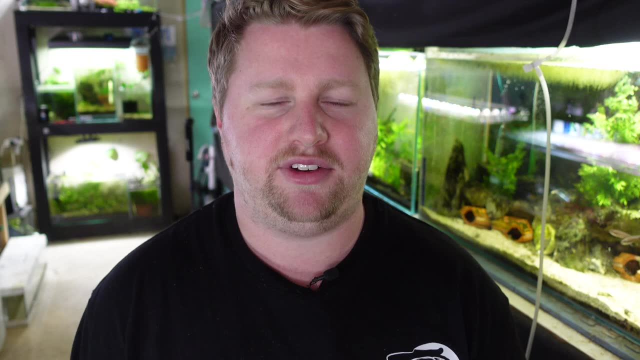 Culturing Daphnia is fairly simple, since they live their entire lifespan within the water column. All you really need is some properly prepared water and some aeration. We'll get onto that a bit further on down into the video, but the great thing to know is it's really simple to culture. 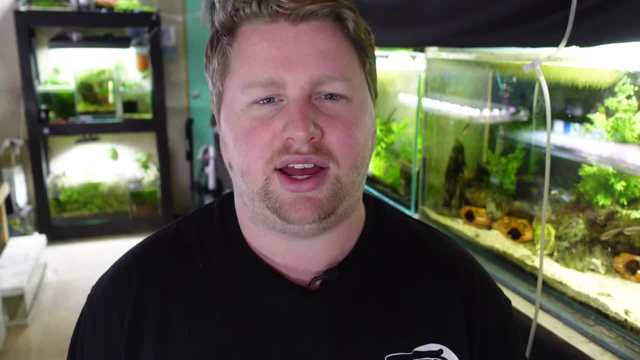 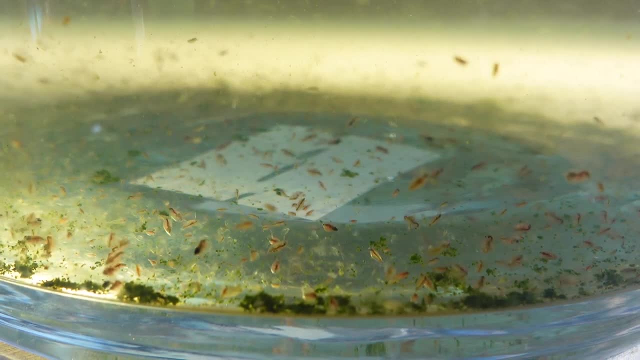 And if you do it successfully and are able to ensure that the culture doesn't crash, you can culture these guys into perpetuity. Things like brine shrimp are a really great live food to culture. however, you do have to keep buying eggs, but something like Daphnia is self-sustaining and they'll create their. 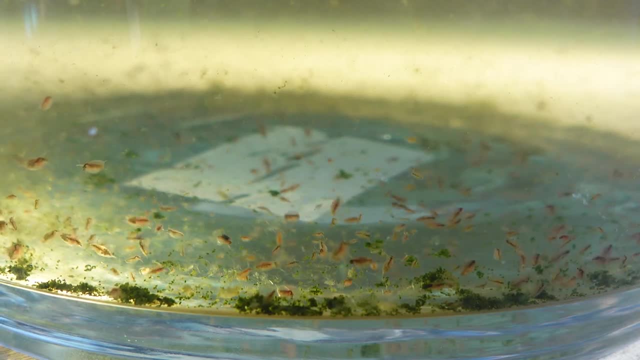 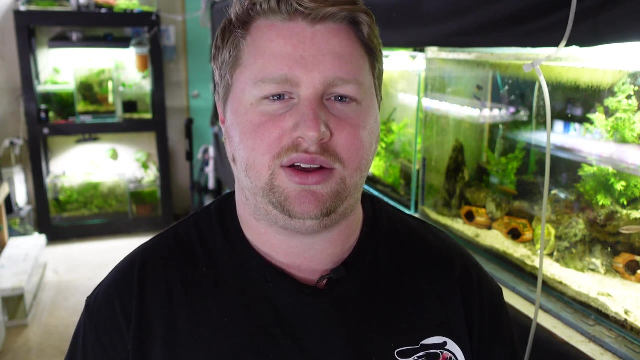 own eggs and their own offspring and live their entire life cycle. in your culture That life cycle doesn't take very long. they're fairly short-lived, only up to a week. but that is where some people do fall down. trying to keep Daphnia is maybe you sit on the culture for a little. 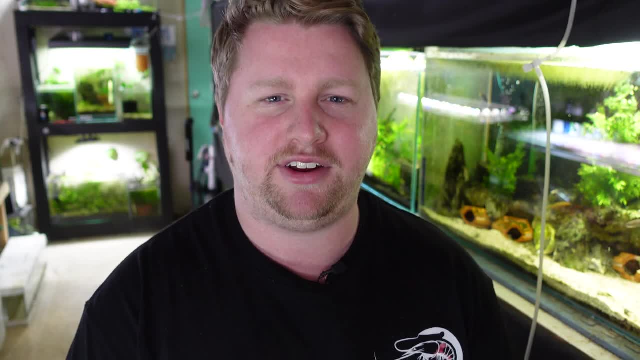 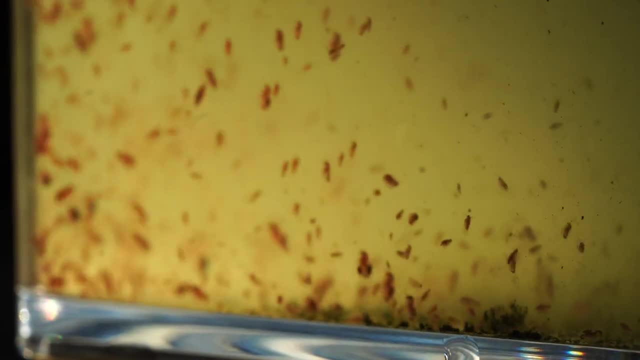 while and you just wait for the population to grow. but this can happen very, very quickly due to that week-long life cycle. so if you forget about them for a few days or a week, the population can very, very quickly multiply and they'll start to become a. 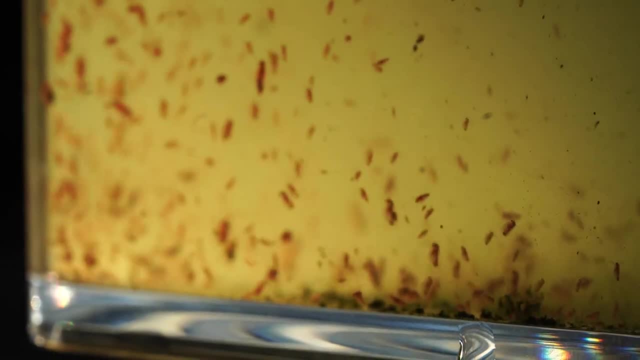 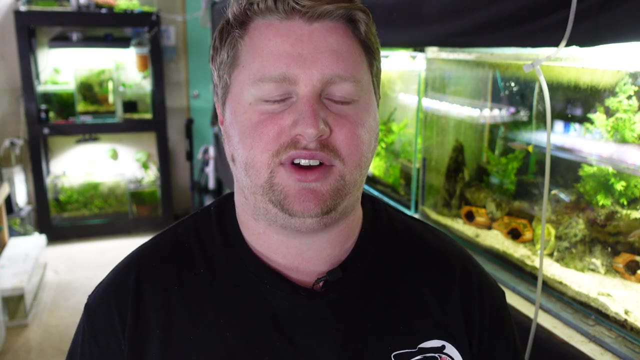 bit cannibalistic and ruin the water quality as well. So that's one area where people can fall down and have their culture crash. Outside of that, if you are able to keep them and have them survive, they'll provide a really great source of carotenoids. 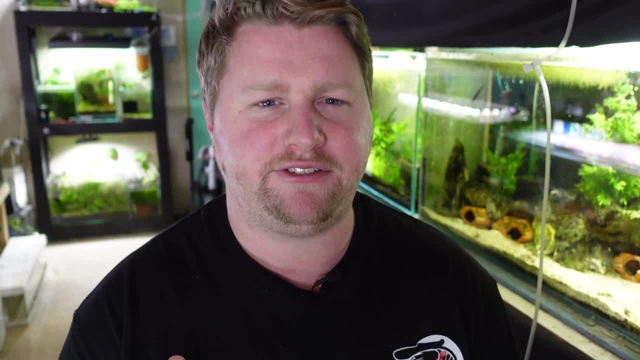 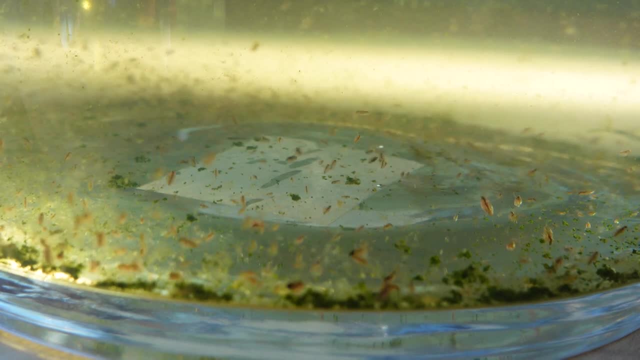 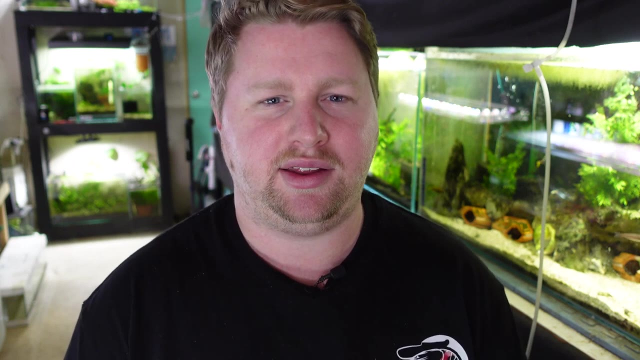 vitamin A and vitamin D to your fish. Carotenoids are great for natural color enhancement, vitamin A is great for development, healthy development in particular, and vitamin D- just like in us- is great for bone development and healthy bones- Three really great building blocks to get into your fish and and. 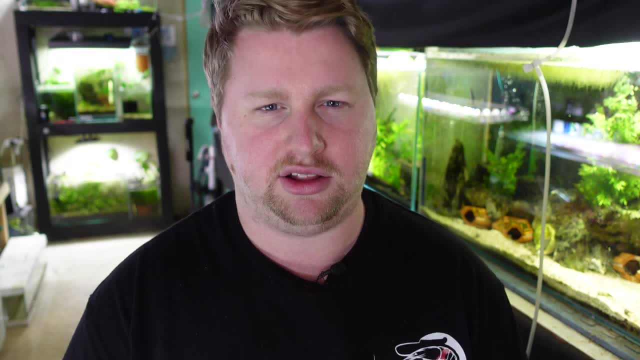 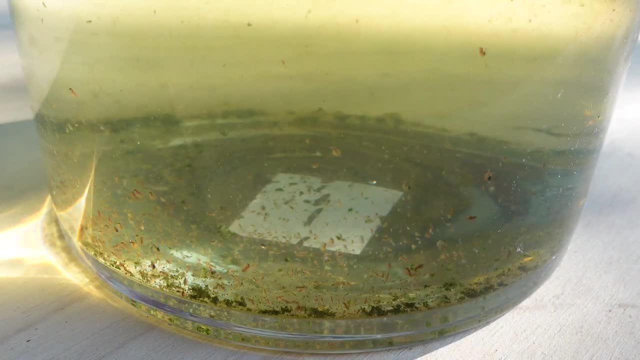 ensure that you have really vibrant, colored, healthy fish in the long term. And the other great thing about culturing Daphnia is you can also culture other things in the exact same tank. You could give it a go of Daphnia and Blackworms, for example, or Daphnia and Amphipods or Scuds. 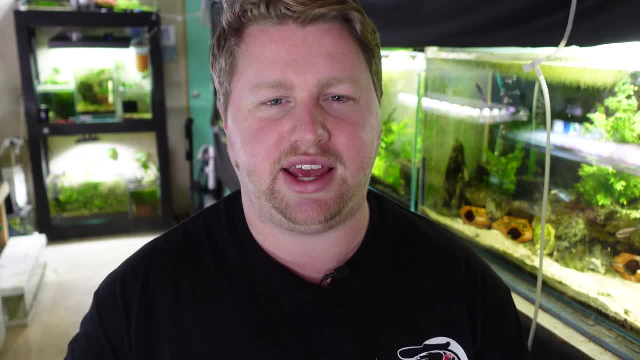 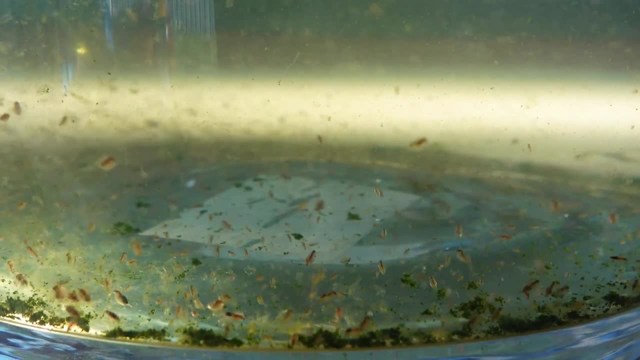 and you can get a really nice mixture going with some great live foods to feed to adult and baby fish alike. So to get started, where do we get our starter culture from? There's three options when looking to procure some Daphnia. First of all, you can buy 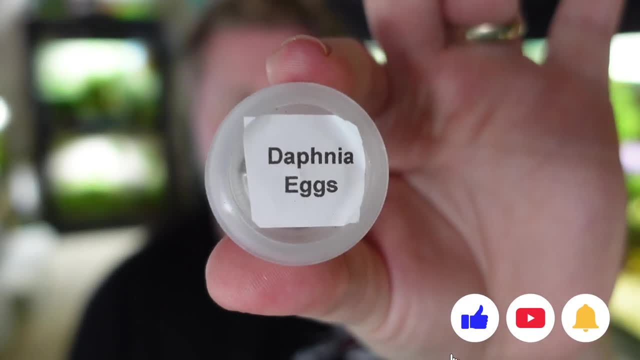 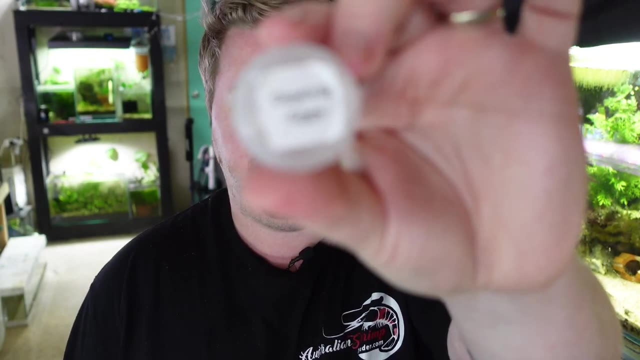 in this Daphnia egg form here. These can be readily found online on eBay or other sites like that, and are fairly easy and cheap. You can also store them, for example. I keep these eggs as a bit of a backup here, so that, if my colony does crash, at least 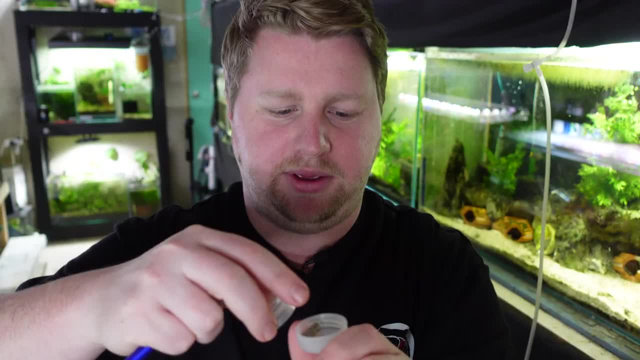 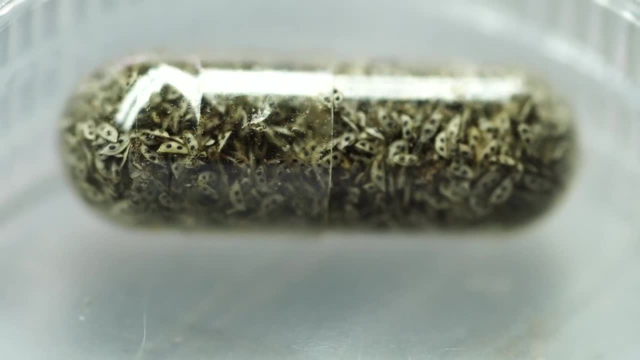 then I can start it up again from here. If I open this up here, you'll probably find that usually it'll be within a capsule. Sometimes they might be loose in a plastic bag or a ziploc bag, but for me I've just got a little capsule of eggs here for a rainy day. 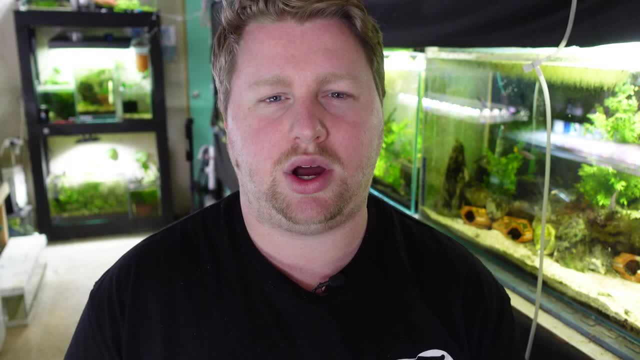 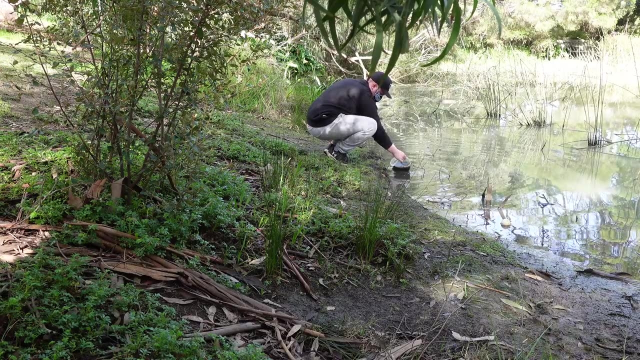 if things do go wrong. The second option is you could, of course, wild collect them if you are from an area that the water doesn't get too cold or too hot. Just head down to a local creek or riverbed, scoop up some muck from the side of it, put it in a jar. give it a week or so to settle and you might see some little Daphnia hopping around in that water. If not, and if you just want to go the easier route and make sure that there's not going to be any other pests or things getting into that culture, like if you were to go and 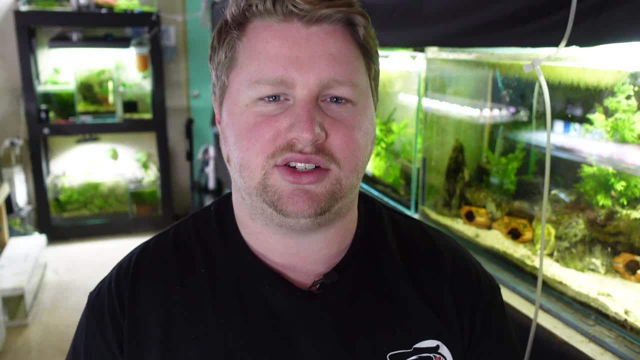 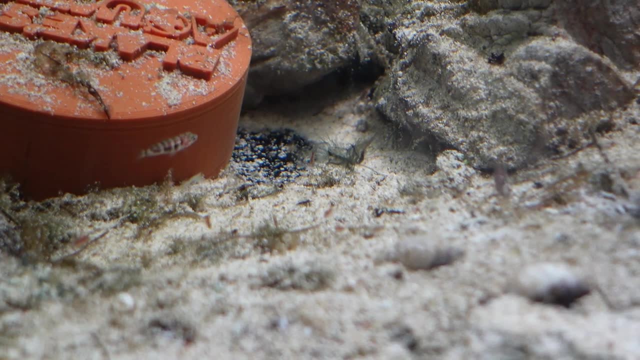 wild. collect it, then you can just pick up a live starter culture as well, And in just the same way that Daphnia eggs are found. it should be fairly simple to find a starter culture of Daphnia, whether that's through another hobbyist or a club or on eBay or another website. 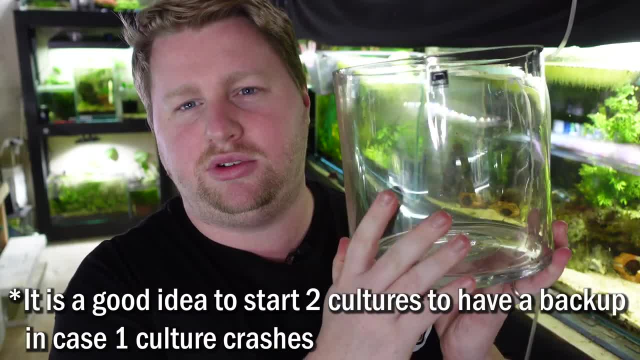 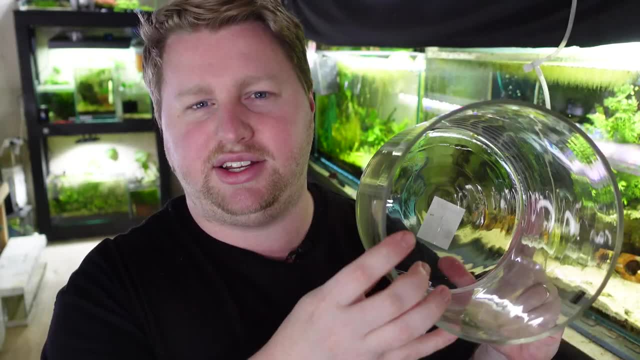 I'd recommend getting at least one fairly sizable jar that you can fill up with water. This guy here is a half gallon or two litre jar here and I'll just fill it up with dechlorinated tap water If your tap water is between seven to. 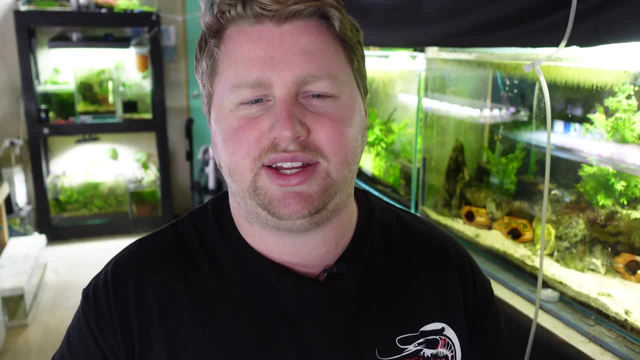 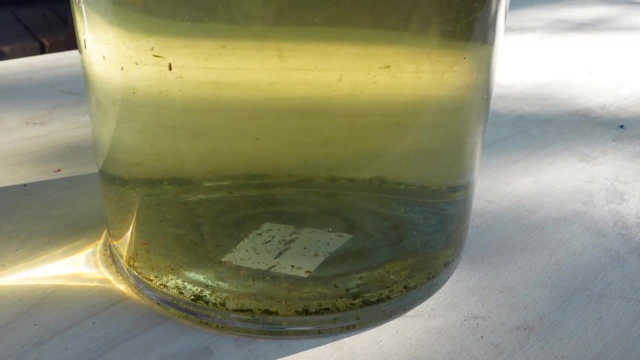 eight ph, then that's brilliant because, just like shrimp and snails, Daphnia do have an exocelaton, which they do shed, so they enjoy a bit of hardness in the water. They'll also enjoy a supplement of calcium which you can provide through, you know, various. 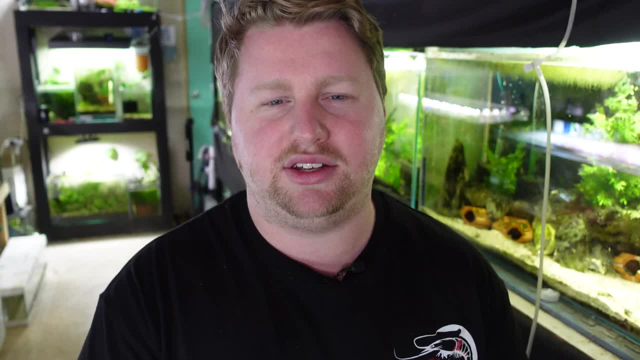 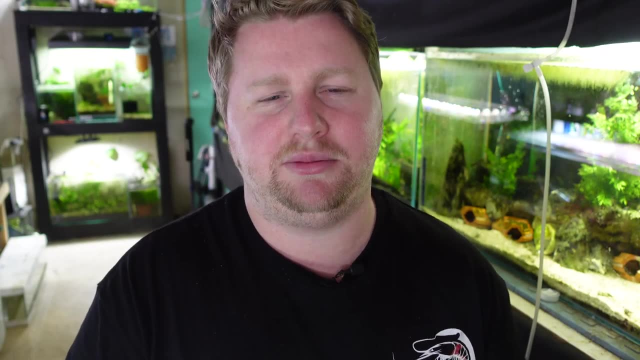 shrimp supplements or also through cow grit, which is typically used for chicken farming. So once we have our appropriate water in here, it's time to talk about temperature, and Daphnia don't really like a temperature too high. As close as you can get it to about 22 degrees celsius or 68 degrees fahrenheit. 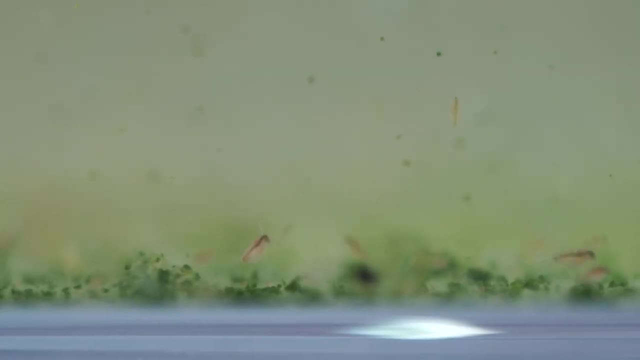 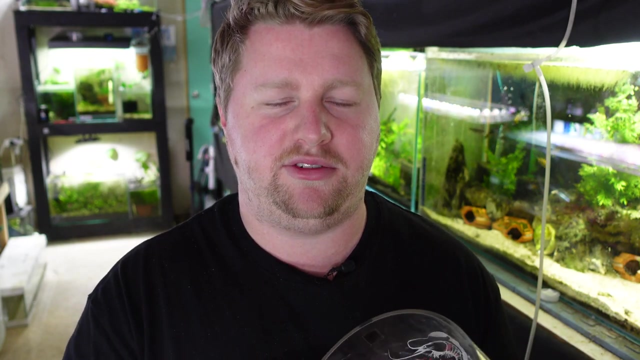 will work brilliantly. I give it maybe plus or minus two degrees either side of that. The last thing that we're going to need is some aeration, and this is a really critical one that I think a lot of people fall over in, because typically, aeration in a vessel like this we're taught that the smaller bubbles are. 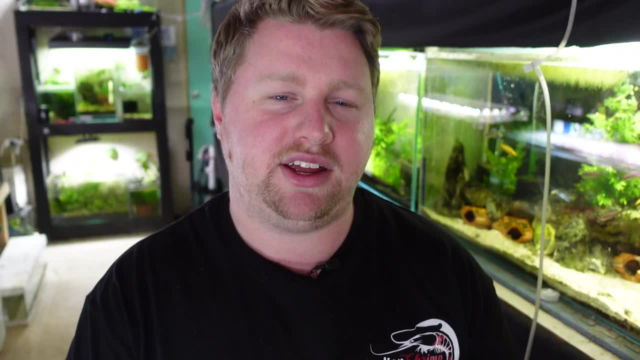 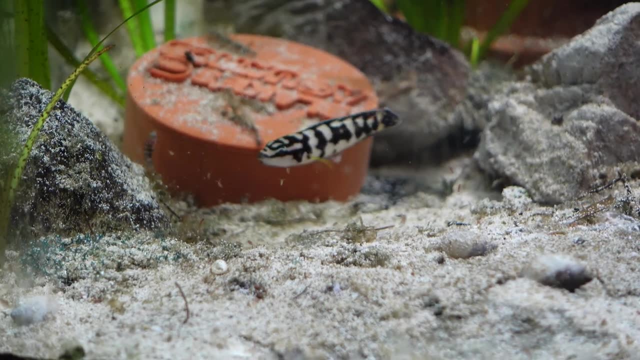 the best because they get the most surface agitation. however, with Daphnia in particular, you want very large bubbles, and that's because small bubbles can get under the carapace of the Daphnia. then they'll be floating all the time. they won't be able to swim properly. 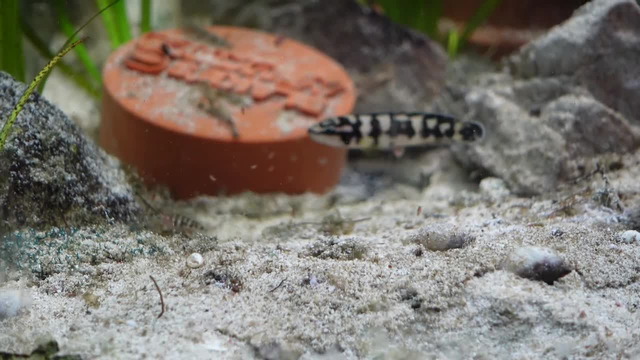 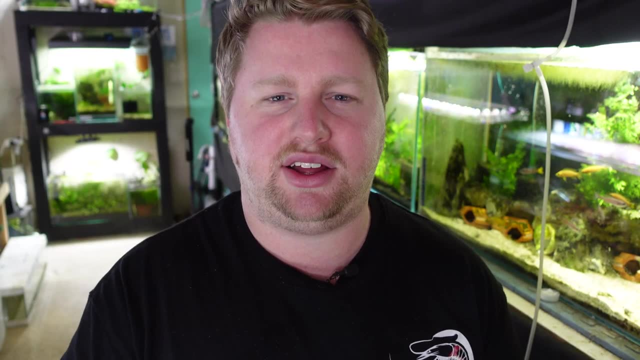 and eventually it will lead to their demise. So we want very large bubbles just to break up the surface area and oxygenate the water. So you can provide that just through a piece of rigid airline or you can just try and weight down a normal piece of airline tubing with a rock or something like that. 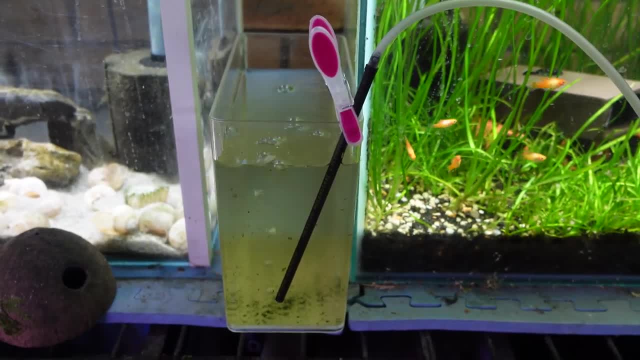 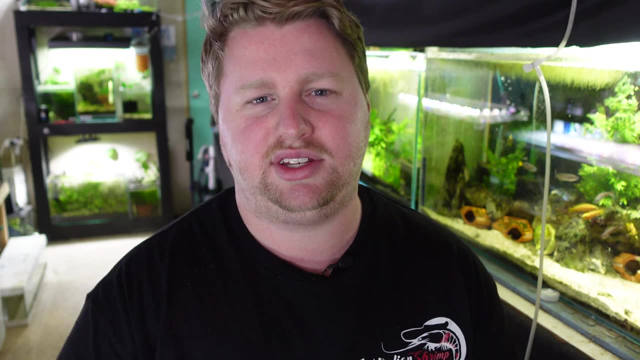 and get some slow moving large size bubbles into the culture. Once we have our water and aeration in our vessel, put our capsule of eggs in there, or whatever your egg sauce comes in, and then it's just a matter of waiting about 48 to 72 hours. 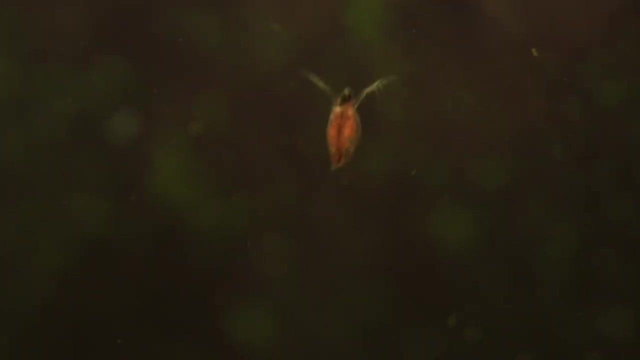 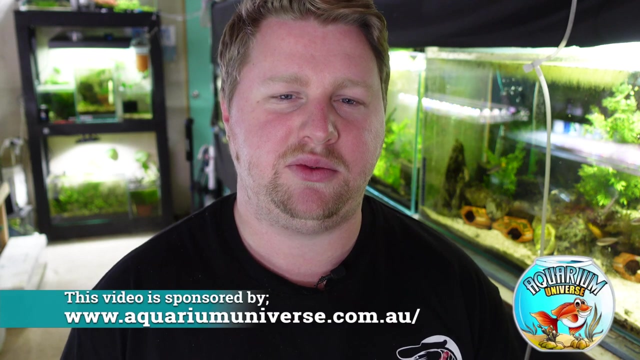 to see the Daphnia hatch out. And once the Daphnia have hatched out, it's time to start to think about what to feed them. The very best food for Daphnia- because they are a filter feeder- is green water. So if you're able to, 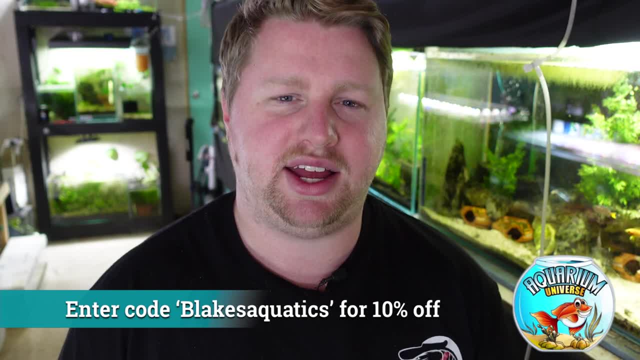 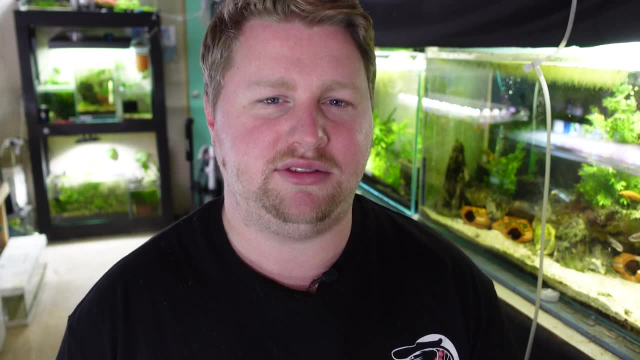 culture some green water by having some water, maybe standing outside or under 24 hour light, then that's going to be perfect for them. but if not, we can substitute this with a mixture of yeast and spirulina powder. So I prepare this just by getting some warm water and some yeast. 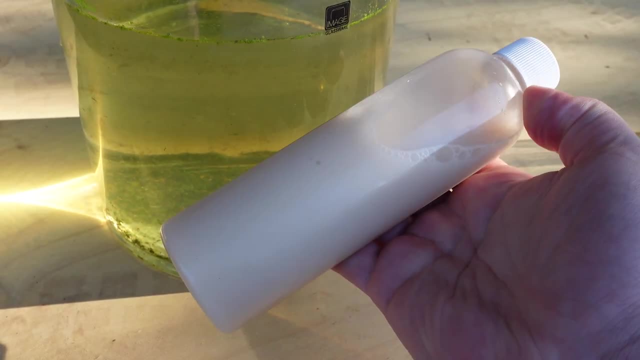 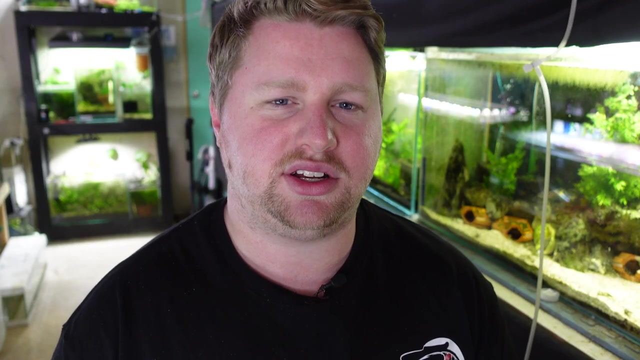 and some spirulina powder, mixing it all up and then storing that in my refrigerator so that I can feed sparingly. I do really want to emphasize feeding sparingly, because the quickest way to ruin your culture of Daphnia is by spoiling it. 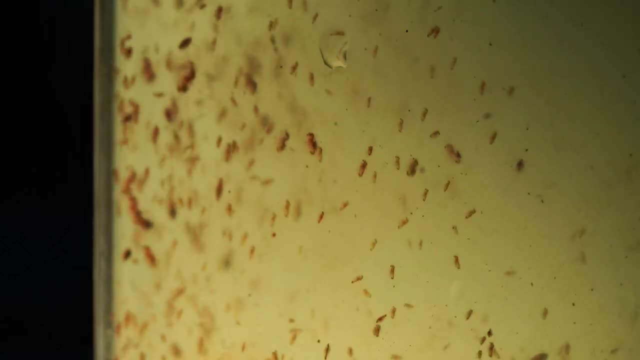 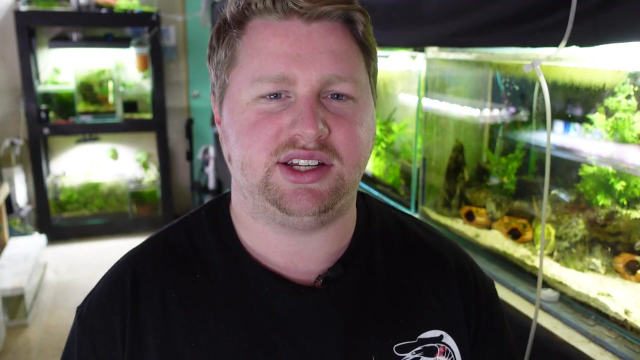 through overfeeding. Keeping in mind that we don't have any filtration on our culture, things like spoiling and rotten food is going to go a long way to ruining our water condition and making it uninhabitable for our Daphnia. The way that I do it is: I just take a small 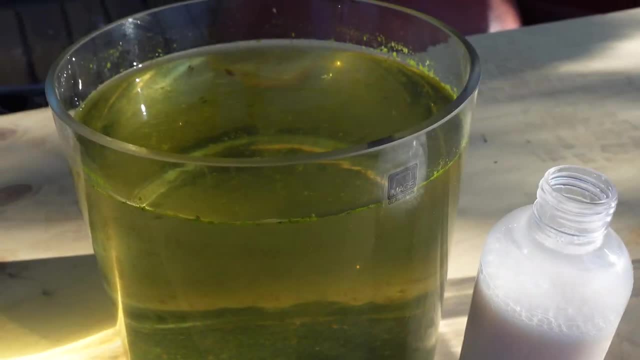 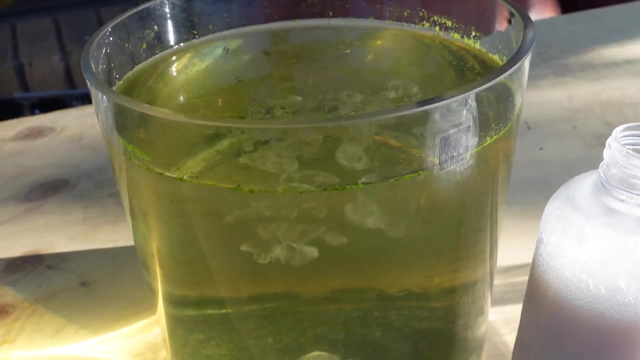 pipette and feed about one milliliter of this, The water will go a bit cloudy. I'll wait for the water to clear up and then I'll feed again. You could also try other types of flowers, like chickpea flower or pea flower, to try and get some food into them. but 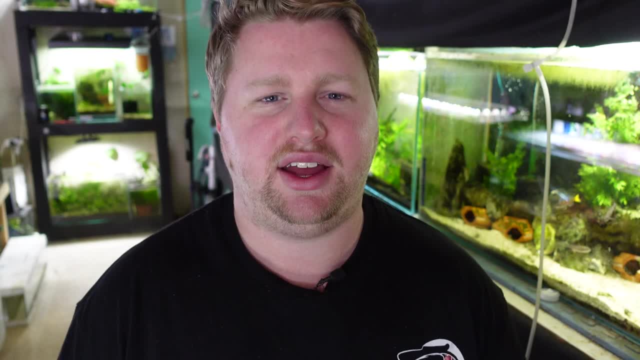 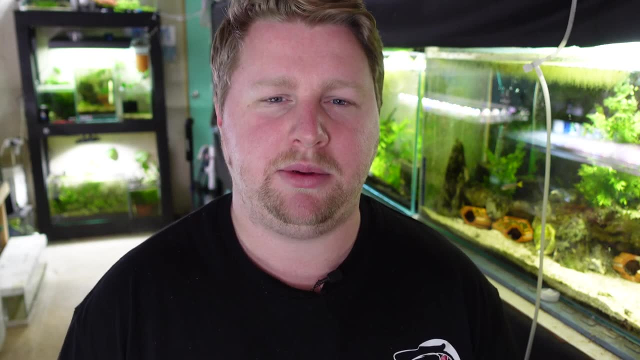 for me, yeast and spirulina powder seems to do the trick. So once we allow our culture to grow and thrive for a few days, then it's time to start to think about feeding out of it. and, just like baby brine shrimp, we are fortunate in that Daphnia are attracted to a light sauce. 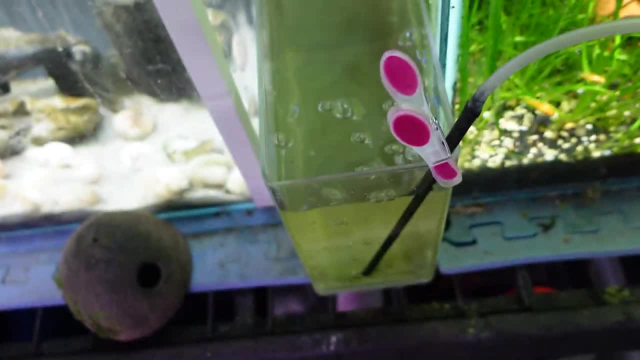 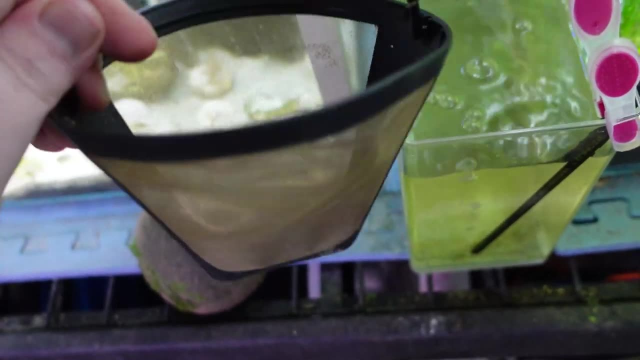 so it's fairly easy to feed them out. All we really need is a fine net, such as a brine shrimp net. I actually have a reusable coffee filter as well that I like to use, and it's just a simply a matter of shining a light at the top of the water surface, scooping up underneath some 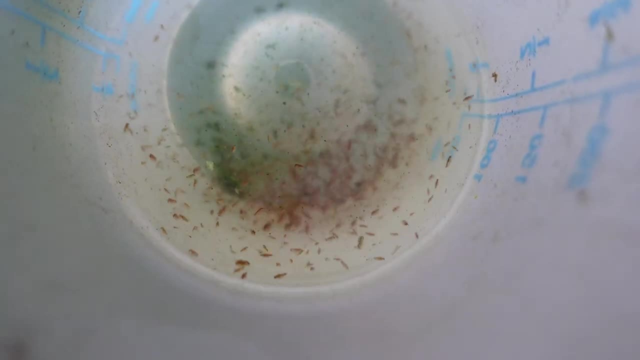 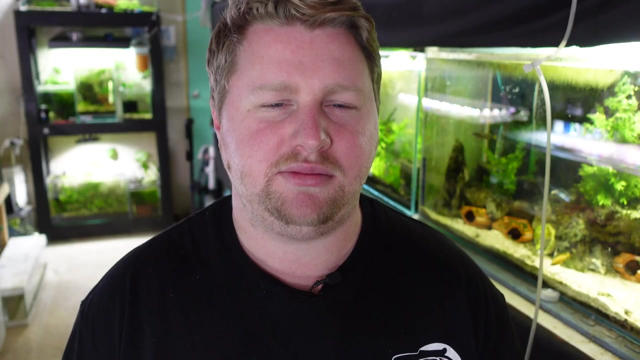 brine shrimp and feeding out just like that. I've found culturing Daphnia to be really, really great, especially for fish like my pea puffers, where typically I've been feeding them live black worms. however, they're a bit shy and the black worms do tend to burrow themselves. 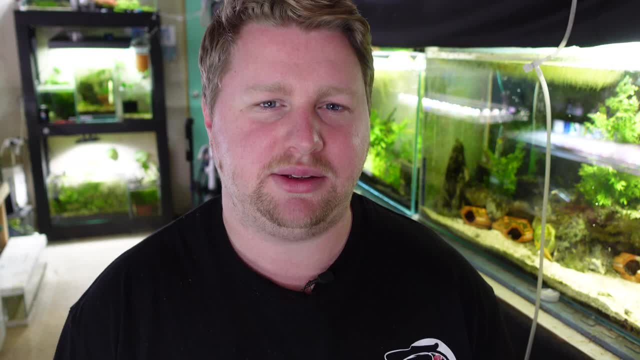 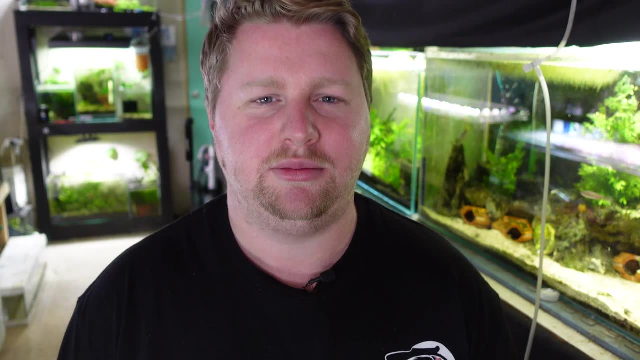 into the substrate before the pea puffers come and eat them. so something like Daphnia that's going to stay up in the water column stay moving around. I can make sure that my pea puffers are definitely going to eat before the food's able to escape. 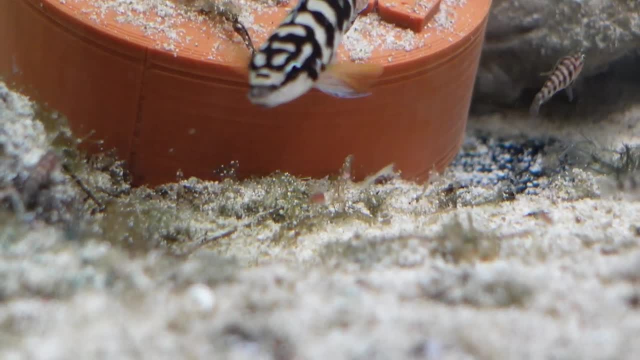 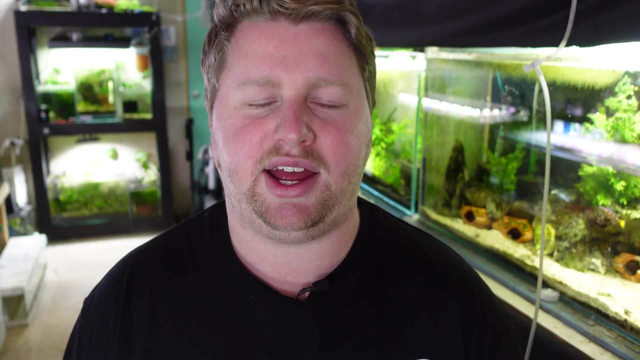 Realistically, the only way that you're going to lose your culture of Daphnia is if it crashes. so just reiterate the importance of don't overfeed, making sure that you are periodically feeding out of there to maintain that colony number, and just make sure that you're not allowing the 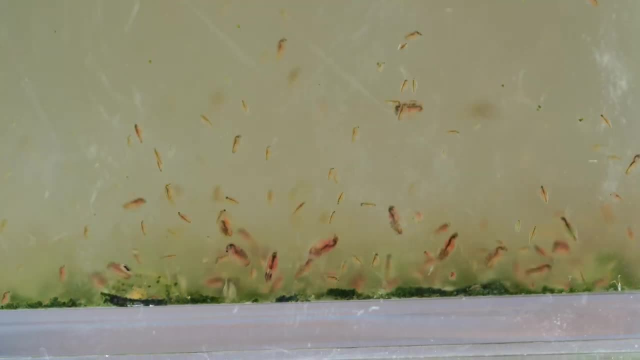 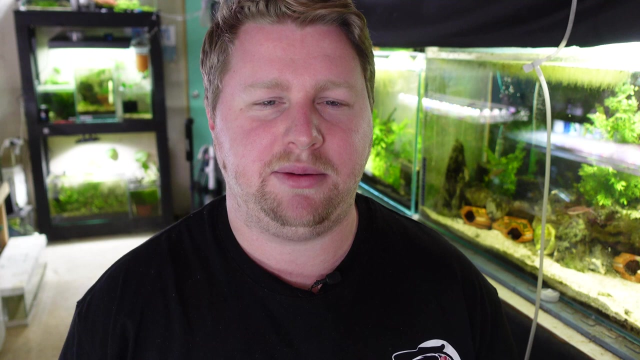 water to get too hot, especially in those summer days. I just want to stress as well: I know some people like to culture their Daphnia outside. it does make it easier to get that green water happening and keeping the Daphnia well fed. however, if you live in an area that gets quite